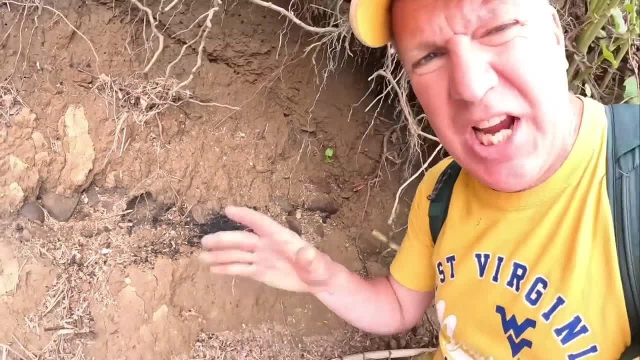 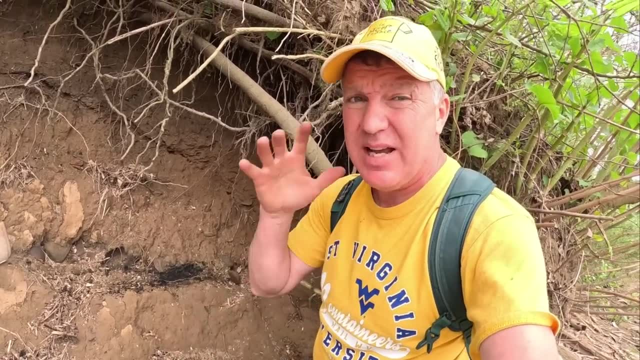 There's a thick layer of charcoal in here too, jammed in with these stones. So what I'm going to do? I got a little trowel. I'm gonna pull some of these stones out and see what we can find. 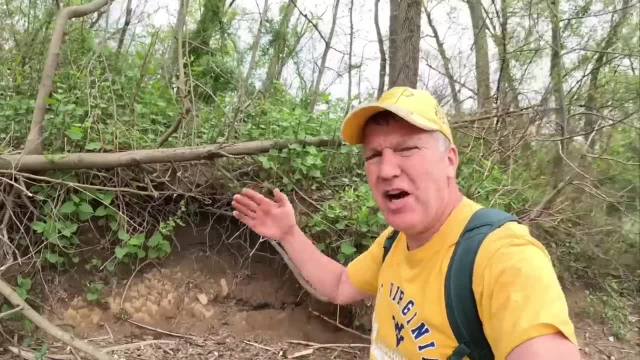 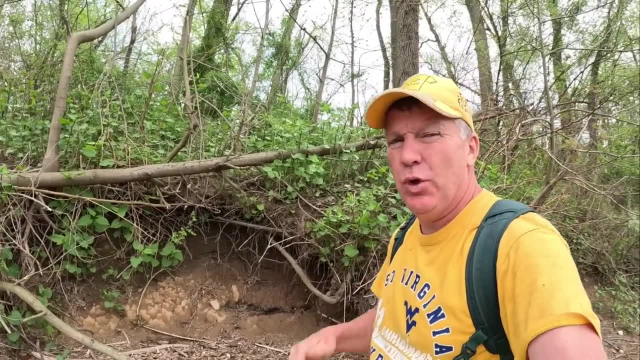 See if any of them are tools or what. And this fire pit is probably, I would say, five to five and a half feet below the surface of the ground up here, which would have been up on a hill at one time, where the natives like to live. 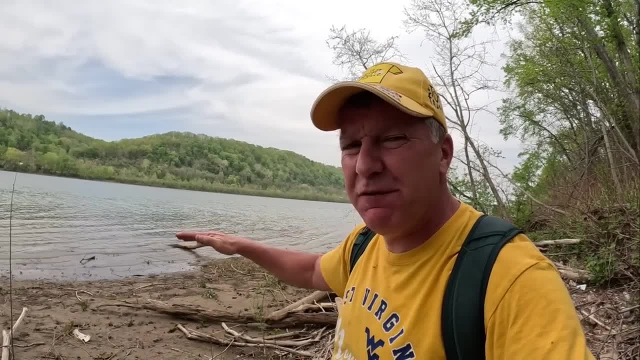 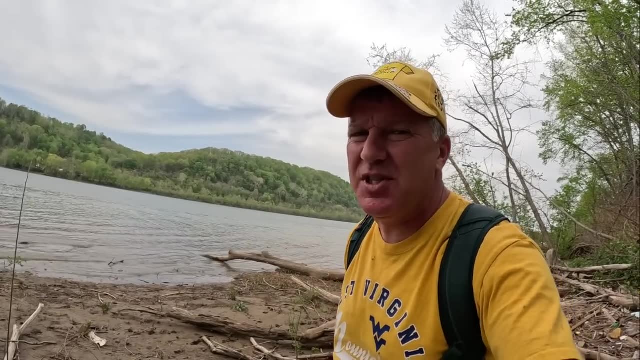 And this Ohio River never used to be this full and before the dams were put in and they were controlling this water, It would have almost never come down here, almost completely dried up sometimes in the summertime, but now when the river floods, it comes up and it eats a little bit more of this bank. up here, where the 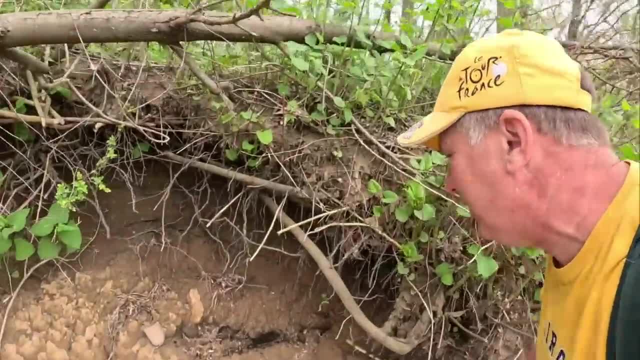 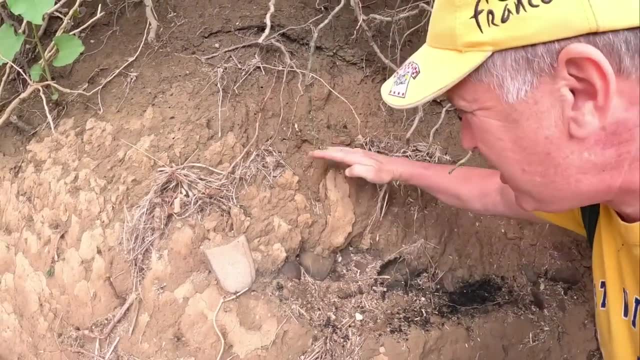 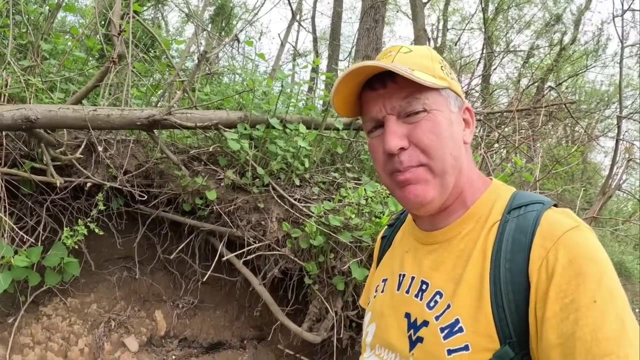 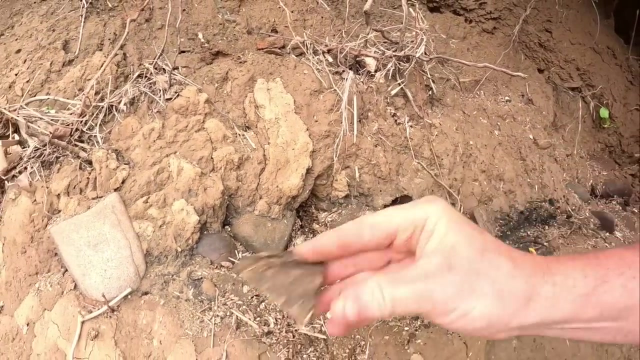 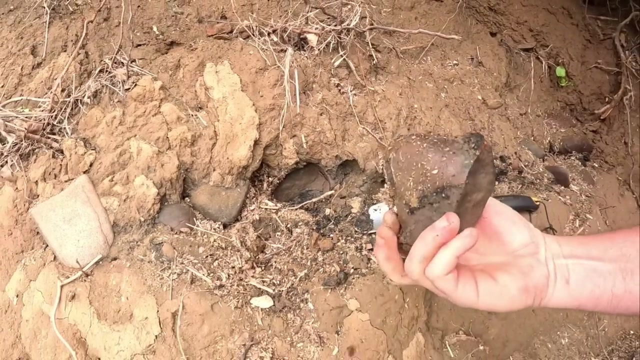 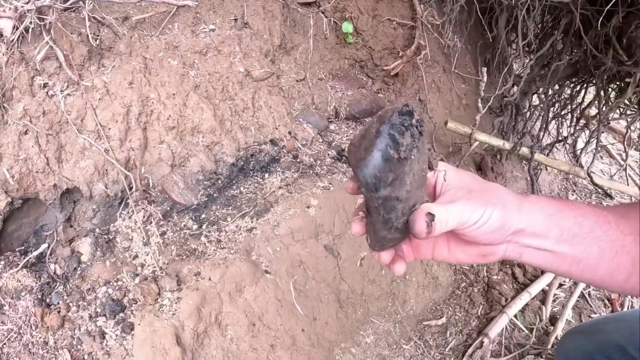 natives were living. and here's something interesting also. you see these fired stones here coming out. these are about 10 inches above the fire pit, so those stones could be people that came in after these folks with the fire pit. these stones are just packed in here. see all that black charcoal coming out of. 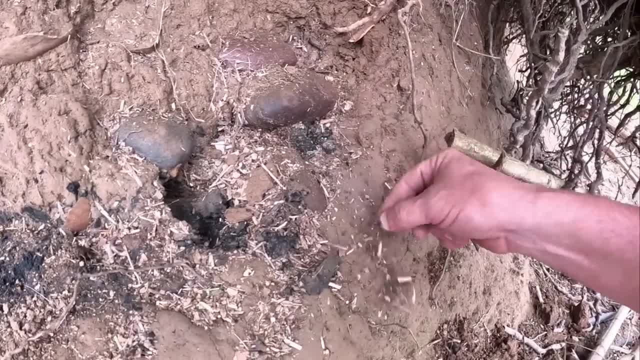 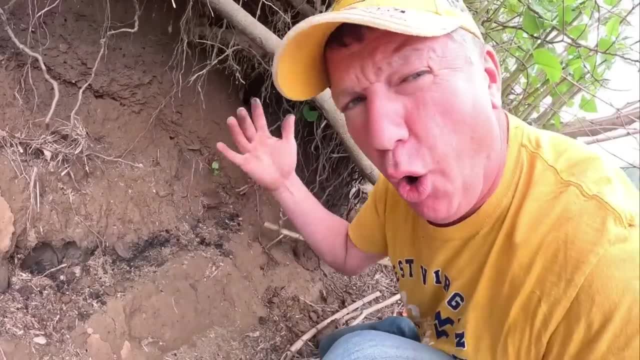 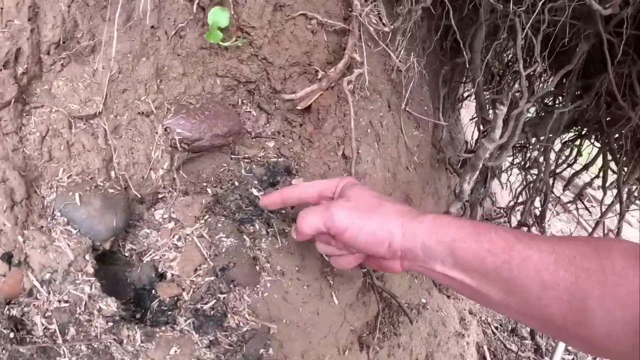 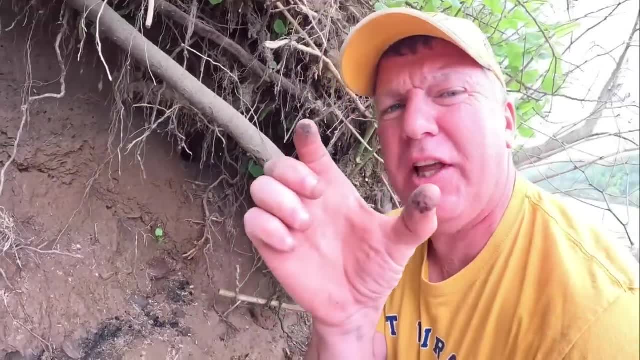 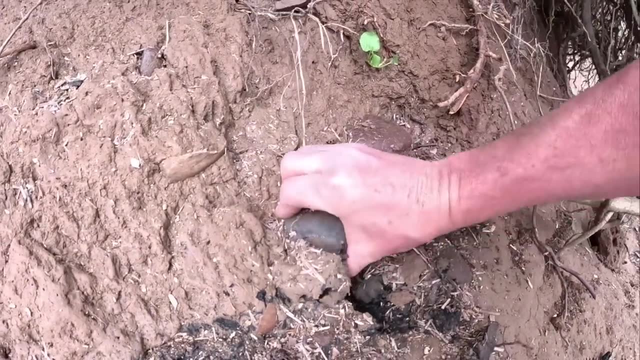 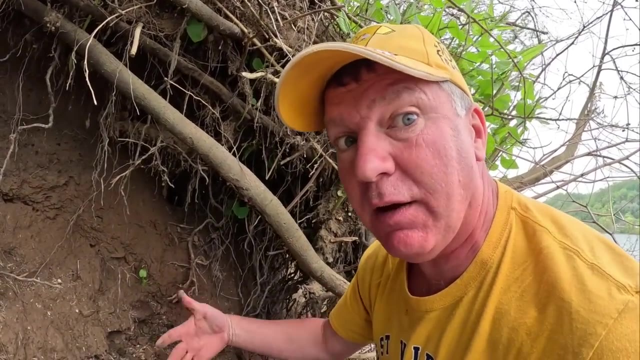 that was sticking out to there. it was like a slither of wood burnt, about that big. this stuff is packed. we're gonna get the shovel and dig a little bit of this out of here and, uh, i'll let you know if we find anything of any significance. 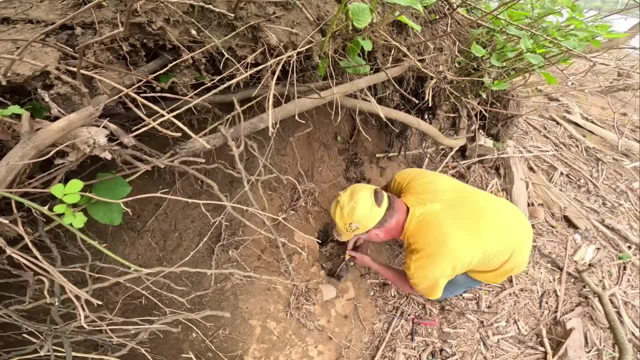 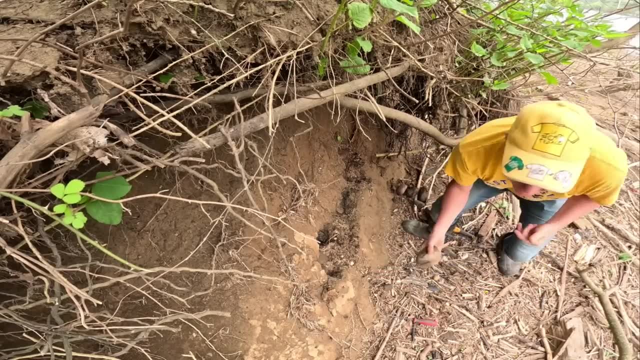 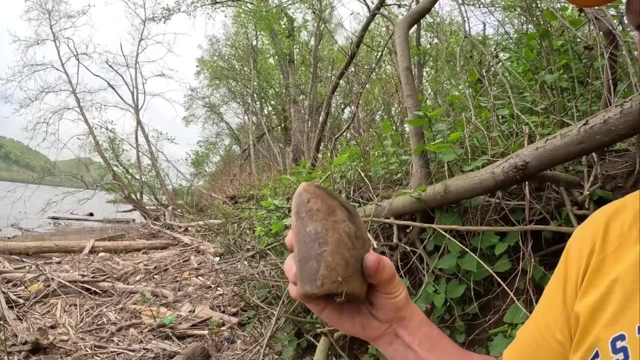 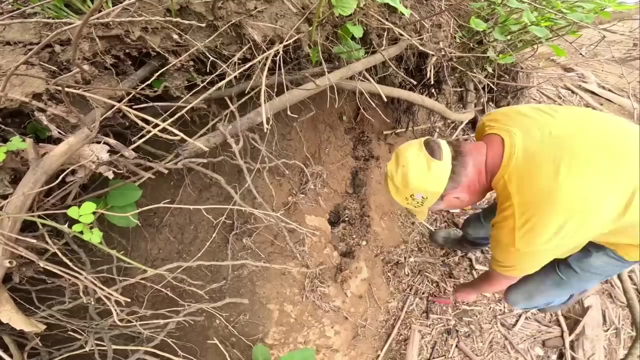 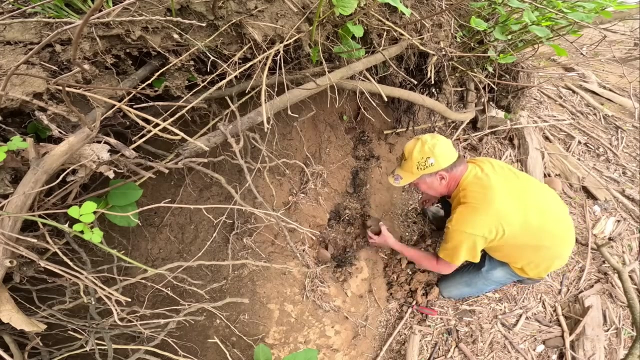 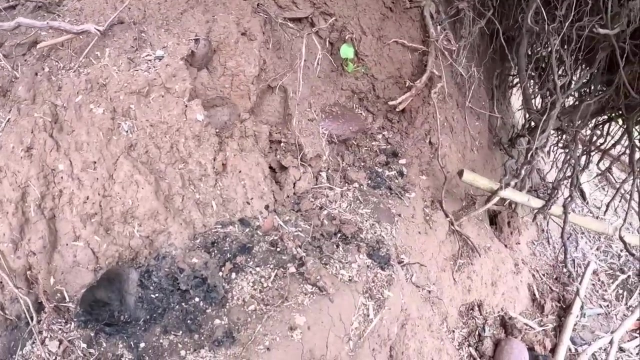 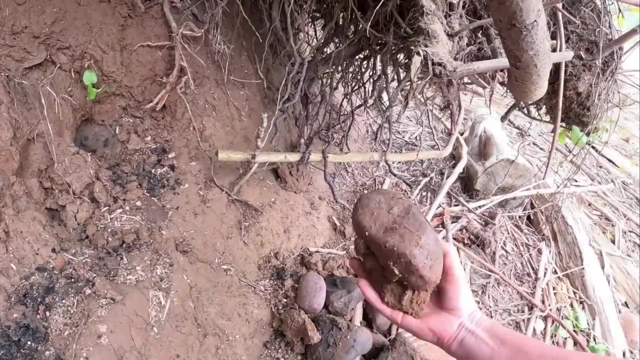 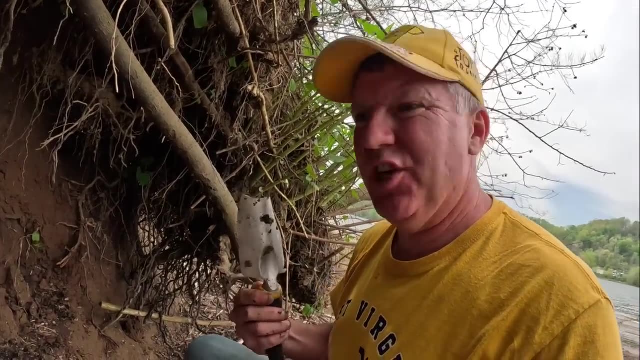 here's half of a grinding stone. you can see this flat place worn on it right there now. it's not quite as nice as the other one we pulled out two years ago, but it is an artifact. let's get back in here. broke my shovel- cheap junk. 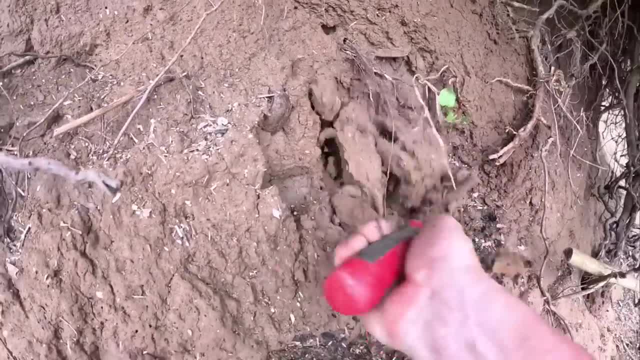 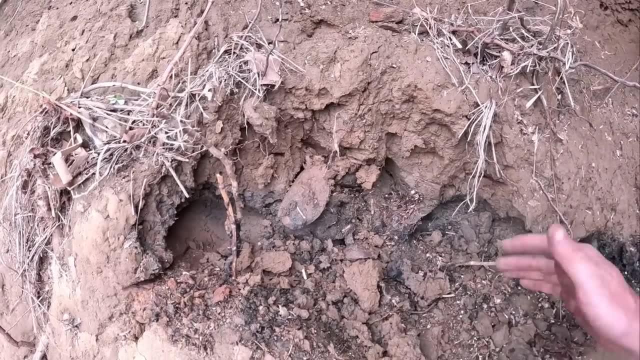 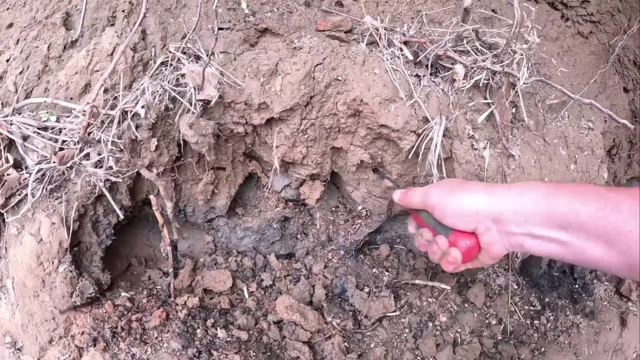 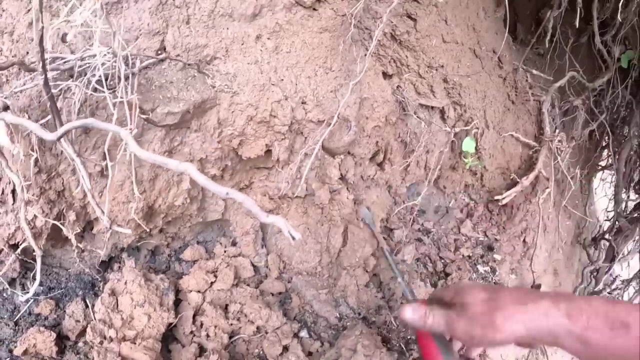 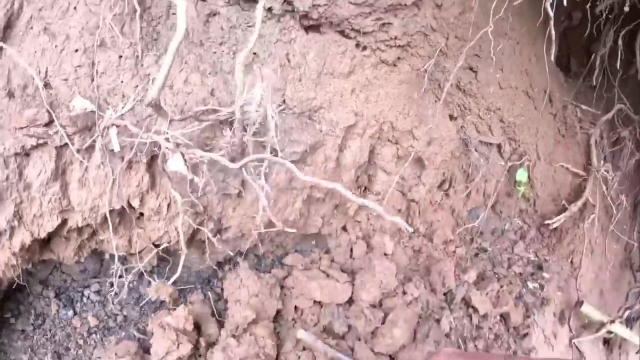 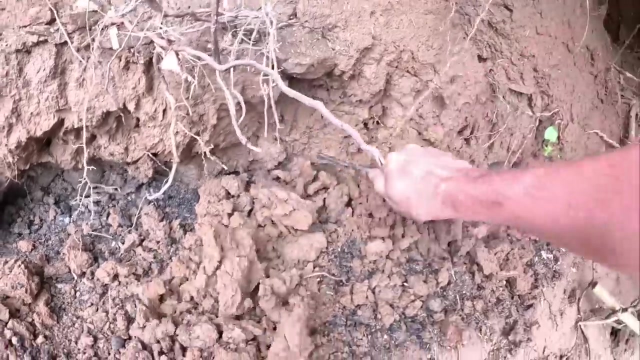 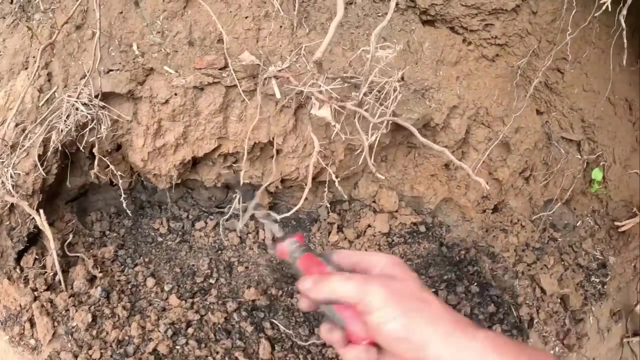 i'm trying to get over top of the stones and then come down into the fire pit so it's not all disturbed when we hit all these uh coals. i think we've reached the back of the fire pit. i got all the overburden off on top. 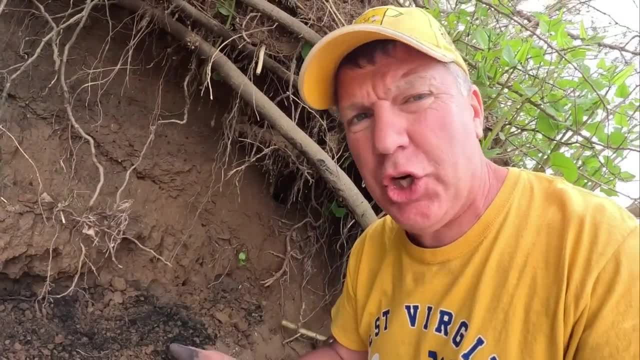 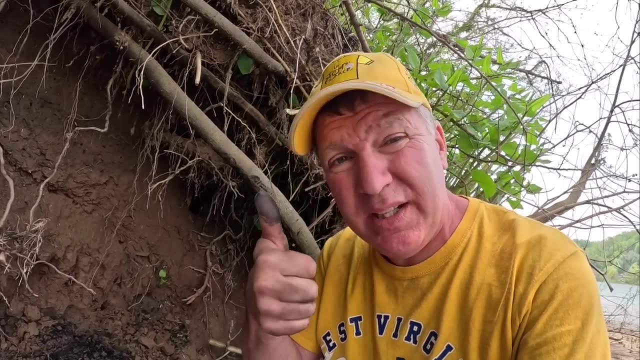 and now what i'm gonna do? i'm gonna sift through these charcoals and see if i can't find any. what i'm looking for is maybe a flint piece, a little arrow tip would be really nice to come out of there. i would know the exact age of it. 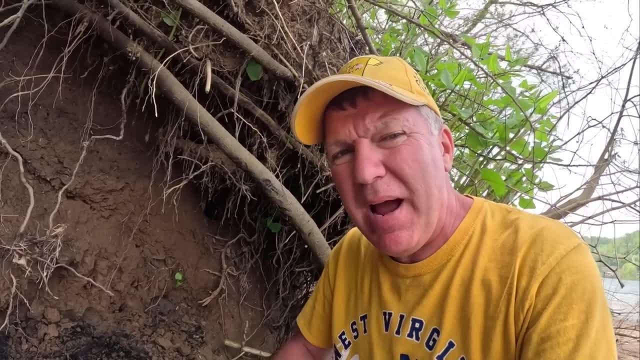 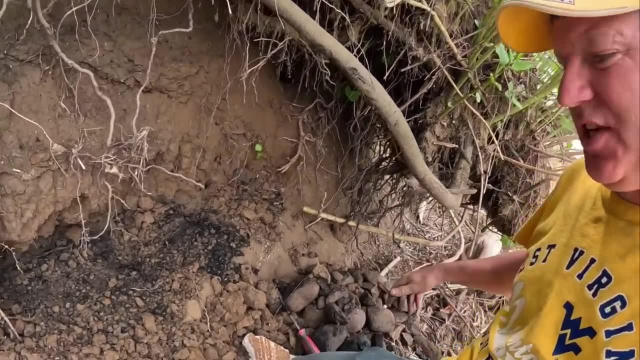 i had this fire pit dated. you can go back and watch the video on that. i'll leave a link in the description below. just to see how old this is, you can see all these stones i've pulled out of here. there's a whole pile of them. 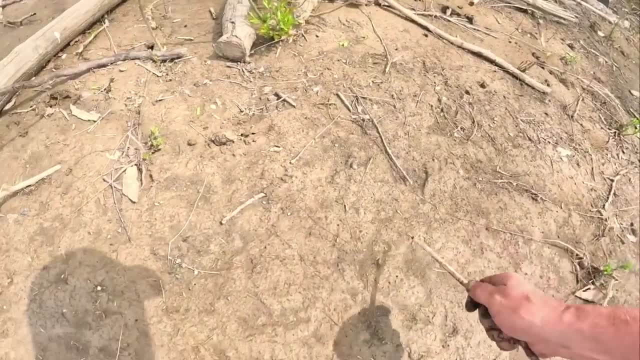 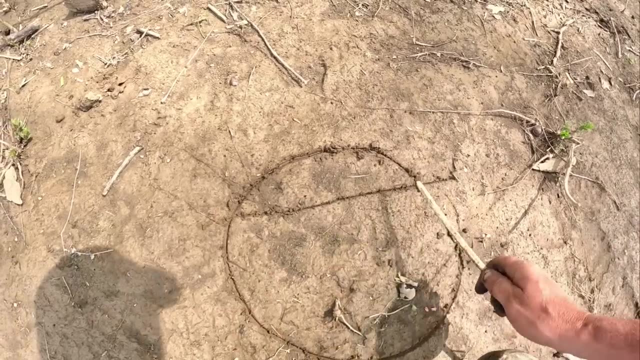 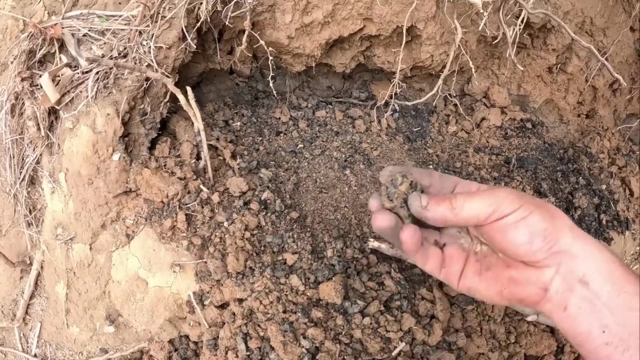 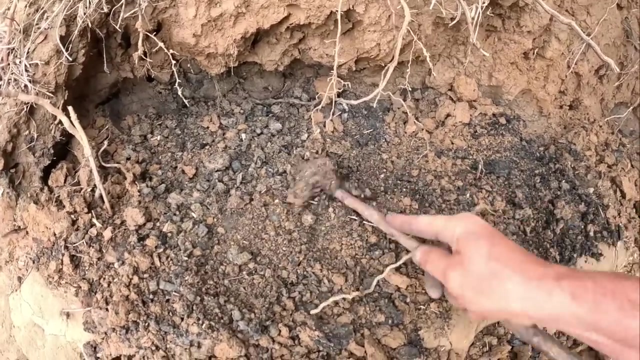 i think the whole front half of the fire pit is gone, like if this was the fire pit. the river has washed it right there and we have wretched the back of the fire pit. wow, these coals are big. that's a huge one there. ah well, 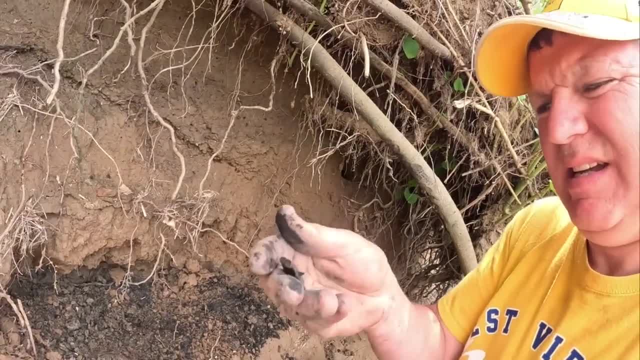 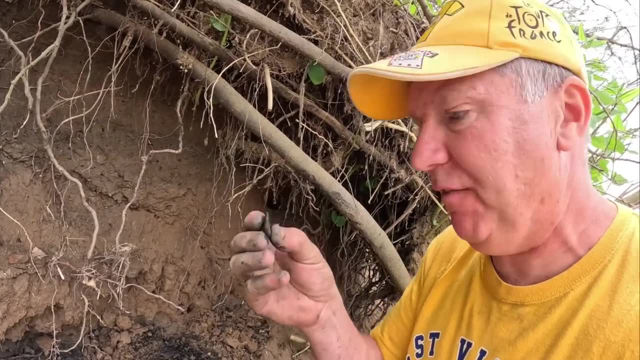 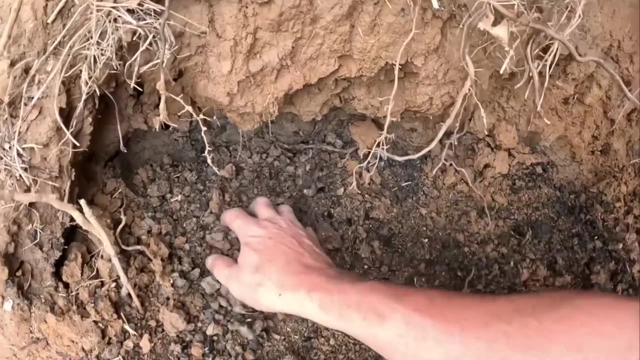 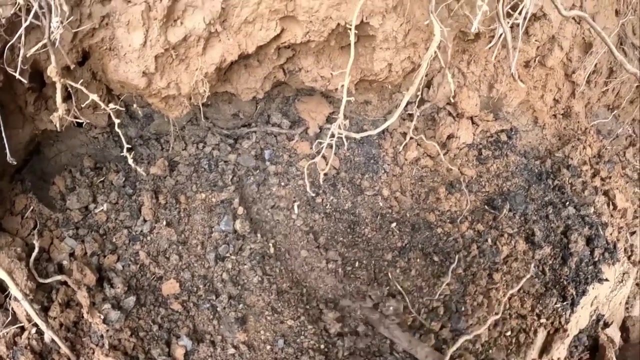 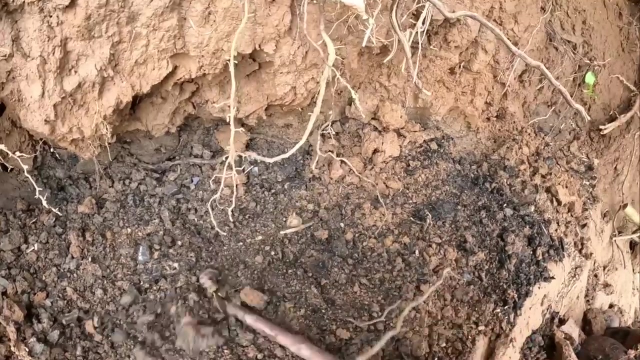 there is flint in here, not an arrowhead, just a piece of debutage, but it is a piece of flint. look at that huge piece of charcoal. whoo stuff's thick in here. this fire was burnt for a long time, i assumed. when they're uh. 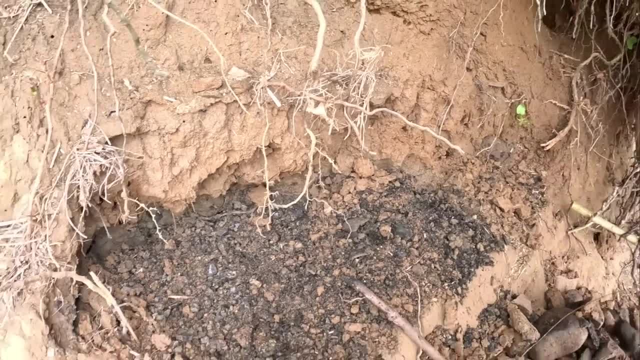 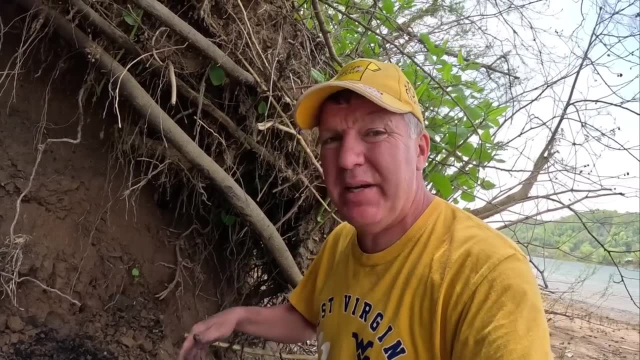 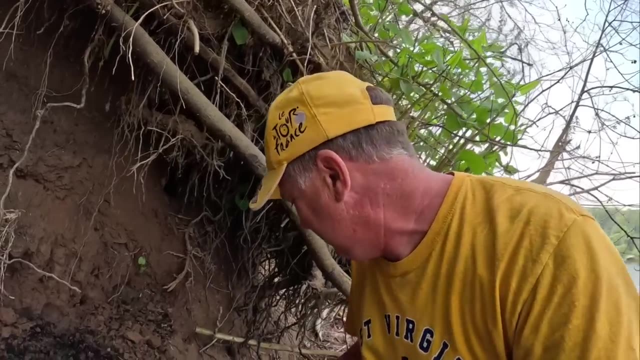 wow, look at that huge piece. oh, that's another rock. my guess is, before they moved out of the wigwam- maybe it was getting kind of run down and they wanted to move to a different place- they threw all the cooking stones and junk in the fire and just left. 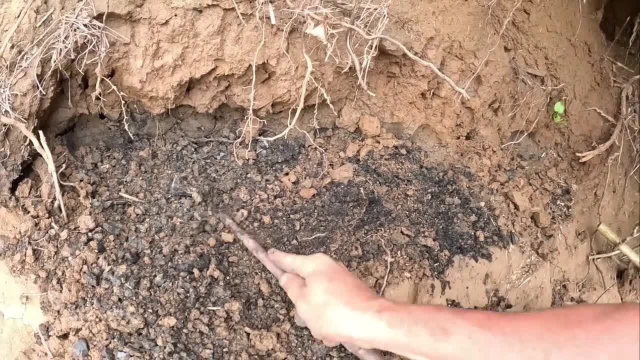 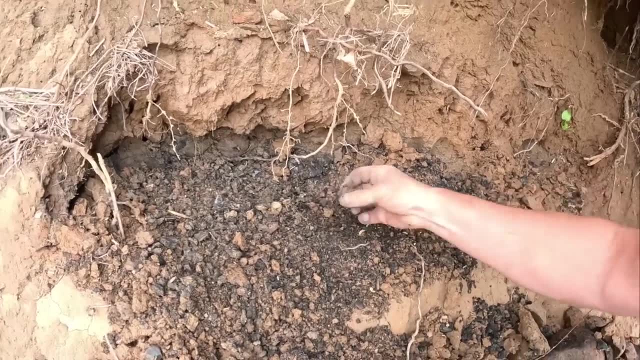 and a? uh. a simple structure like a wigwam. once it was abandoned, it wouldn't have been there two, three years. it would have been rotted down and covered up by foliage. then, with the river flooding every now and then, it's got this under five, five and a half feet of earth. 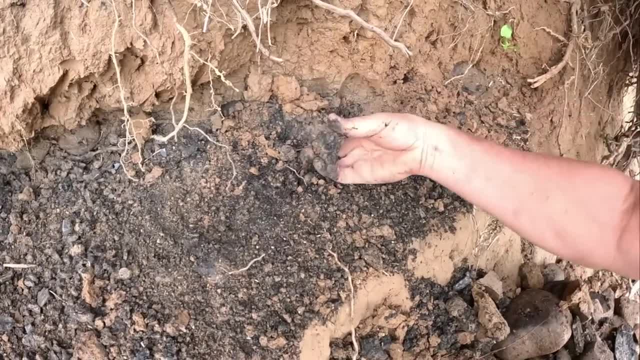 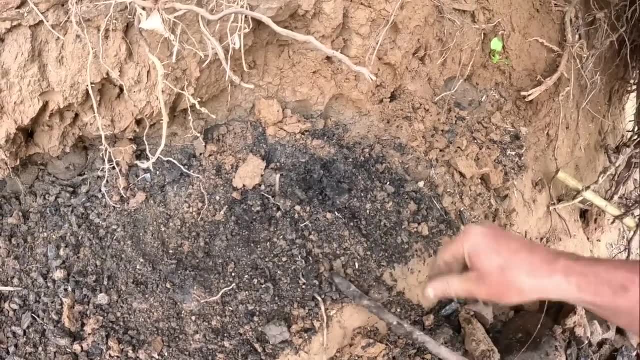 oh, look at that, that's a big rock. look at that, wow, some of these charcoals are huge in here. right, there's a gets thick right there. oh man, that's like a whole, most a whole- branch. you can still see the wood fibers in this. 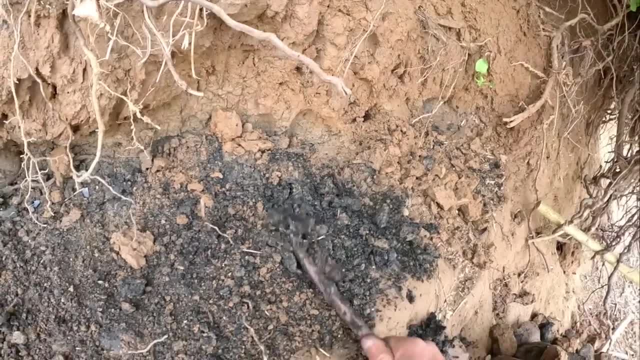 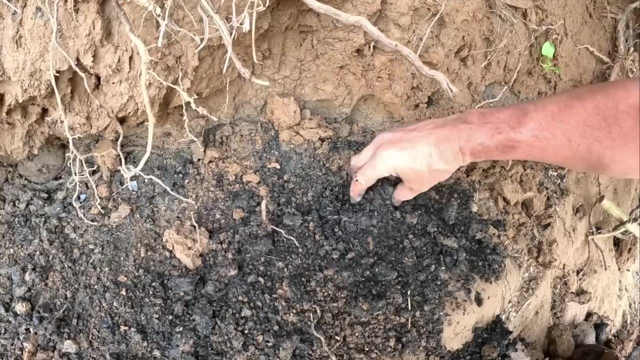 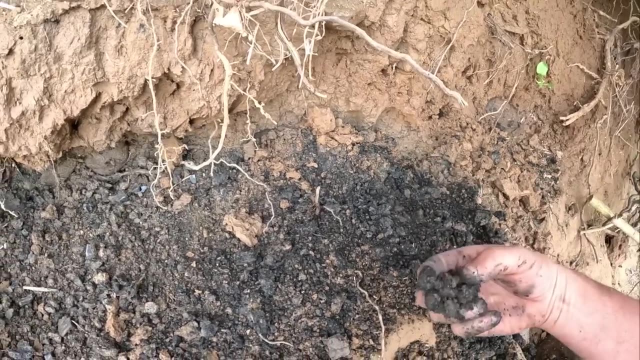 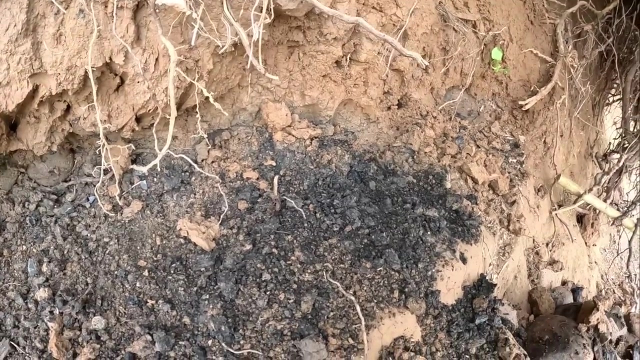 i'm trying to get some of these things out of here whole. some of them are pretty solid, like that one. there was one about four or five inches long, but it fell apart because i kind of squeezed it a little too hard. oh, there's a huge piece. 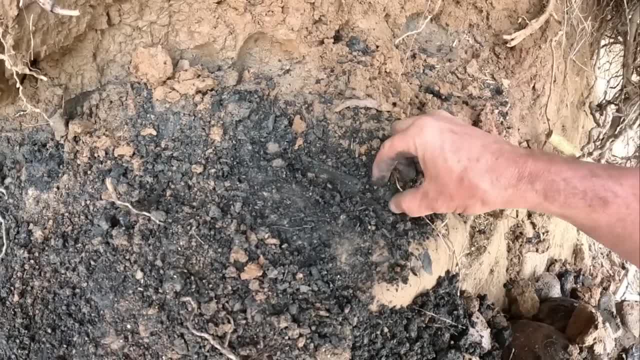 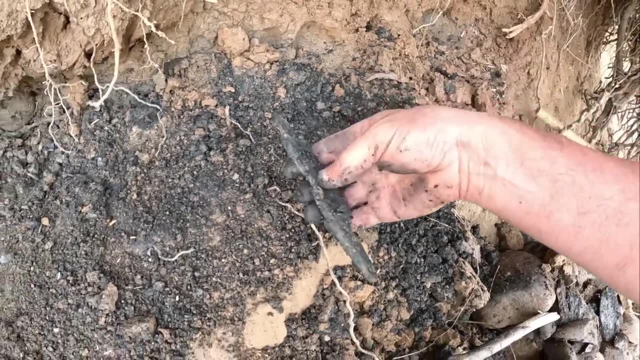 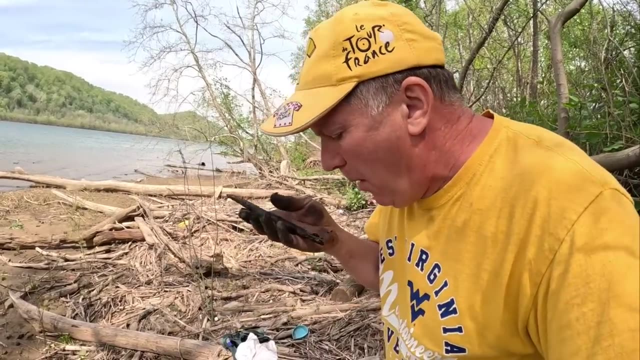 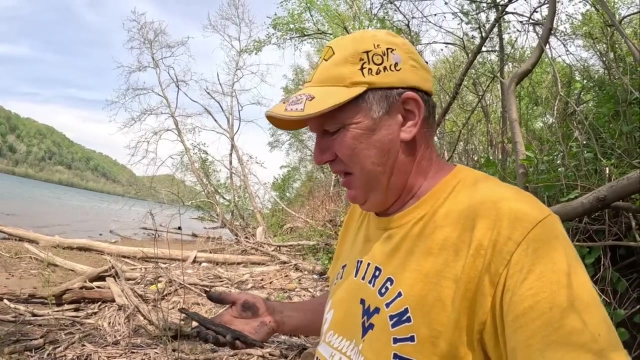 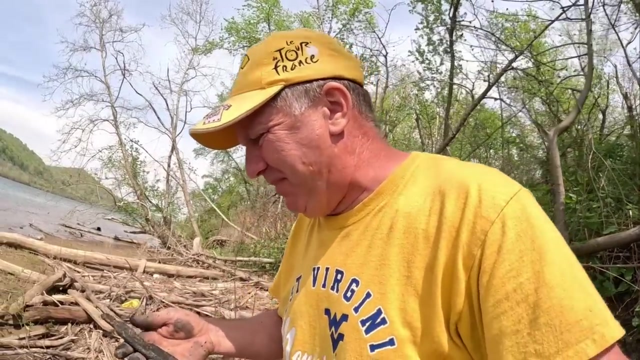 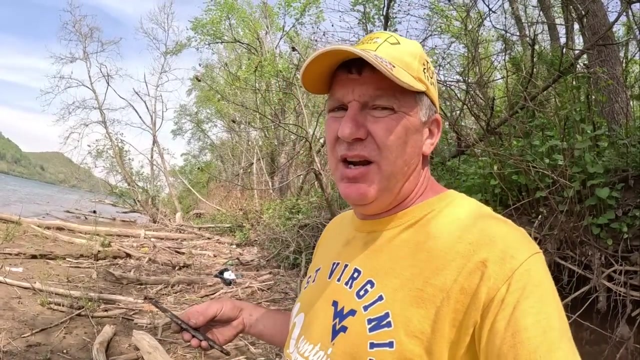 now that one fell apart. oh, look at this like a whole branch. oh wait a minute, hold on, hold on. y'all ain't gonna believe this. my heart just about stopped. now i'm gonna let you be the judge on what you think it is, because i know there's gonna be somebody in there that says it's just a stick. 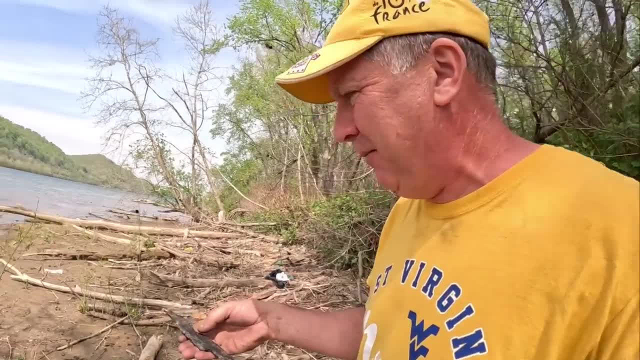 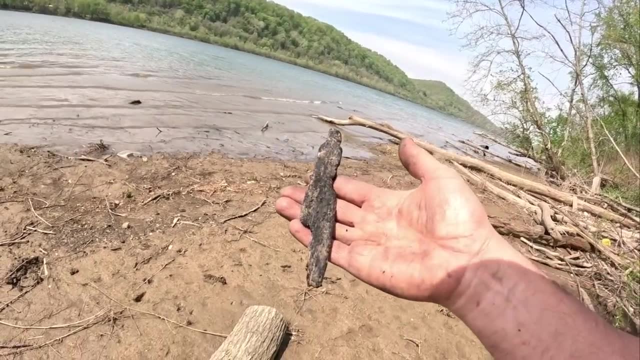 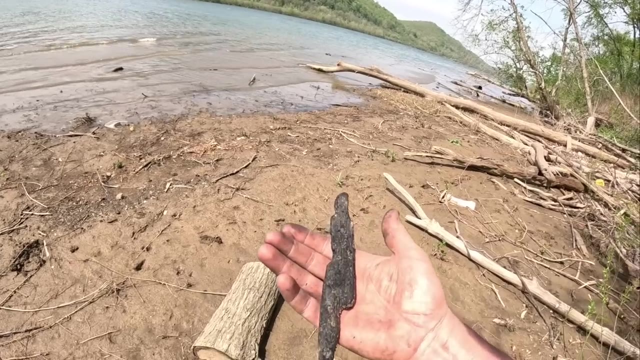 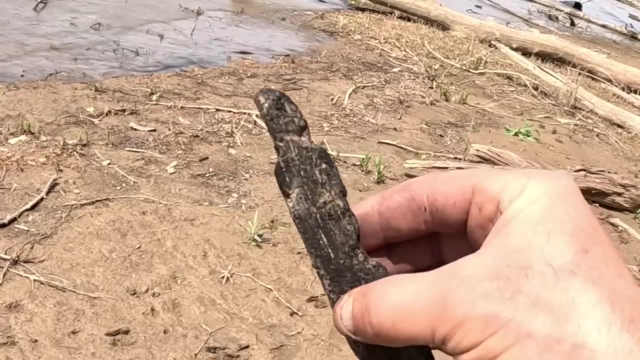 but i guarantee you this ain't just a stick. look at this. let me get you in the Sun. it's very fragile. I'm afraid of it falling apart. I'm gonna have to hand carry this thing out of here, but you can clearly see up there on the top. that's a definite notch, in my opinion. it's what's left of the. 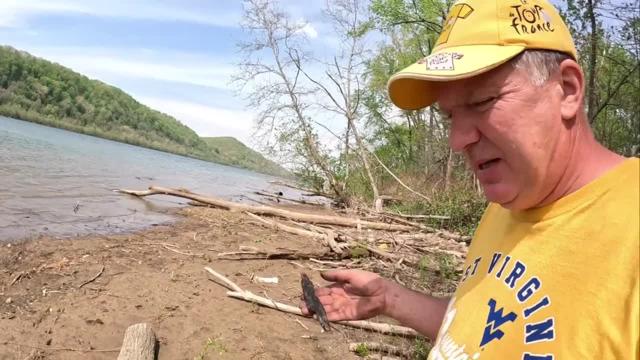 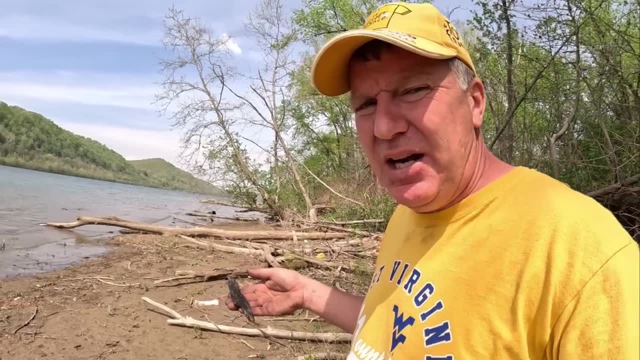 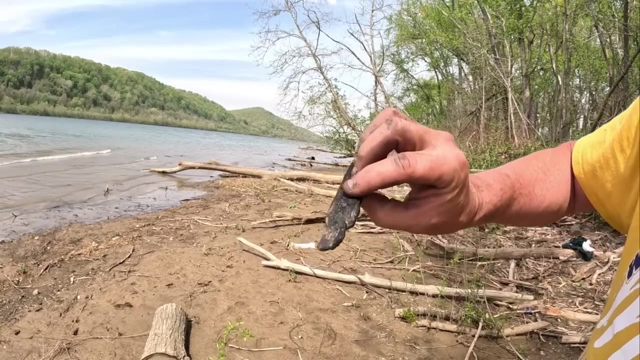 limb of a bow. I'm gonna let this dry and maybe it won't disintegrate or break in half and I'm a hand carry it out of here, but I want you to look at this. you can clearly see a notch right there for a string. and look at this. 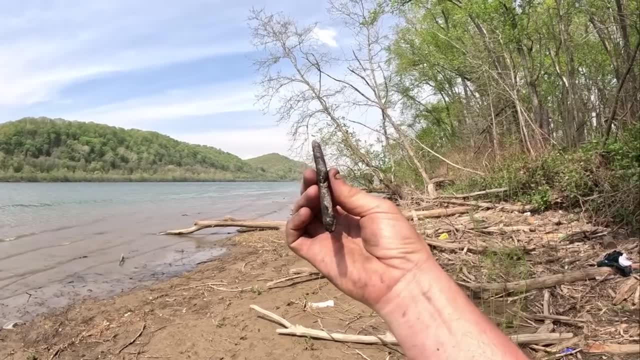 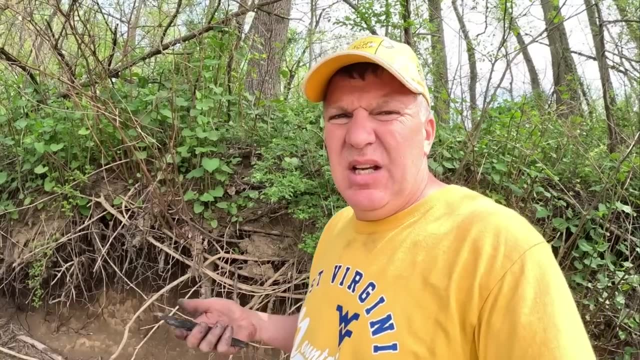 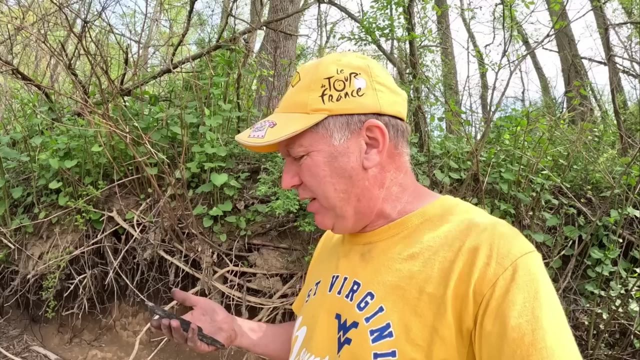 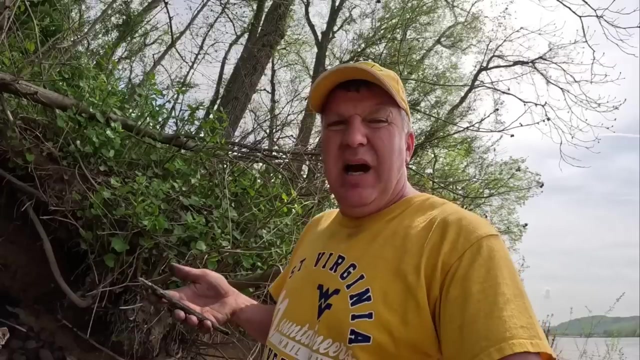 it looks like it's got a slight curve to it. this is the most amazing thing I've ever found in my life. you just don't find this biodegradable stuff around here, unless it's in, like a shell, dump preserved or, I guess, in a fire. now I'm gonna let this dry out. the rest of the 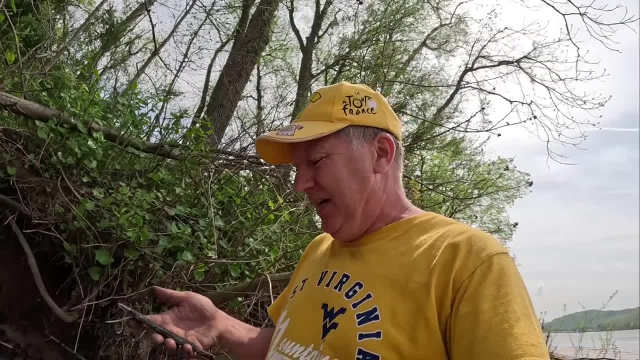 way and then I'll take it home and take a light brush and try to get that dirt off of it. I'm gonna let this dry out the rest of the way and then I'll take it home and take a light brush and try to get that dirt off of it. 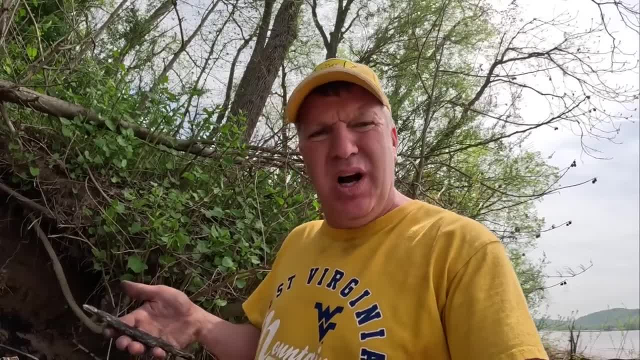 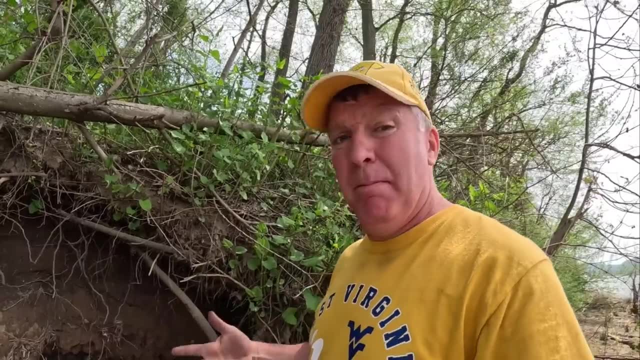 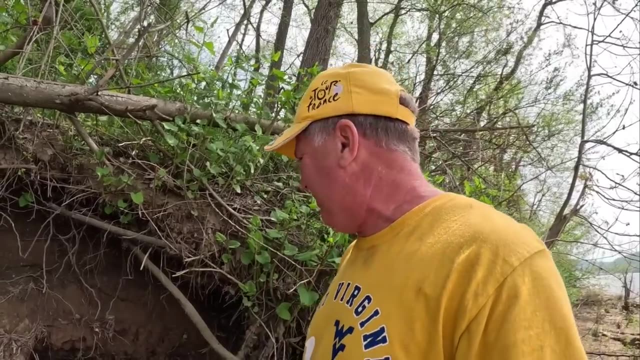 a little piece broke off of it. you can see it's all chipped up. the only thing I can figure is maybe the middle of the bow probably got burned up, but the limb was close enough to the edge of the fireplace when the fire went out and it.